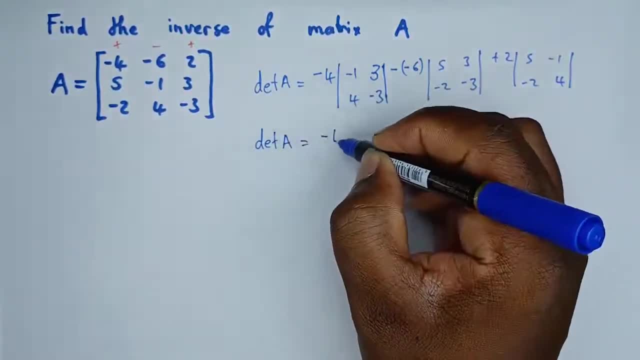 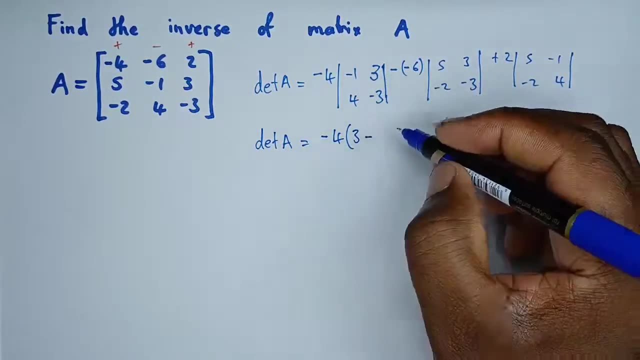 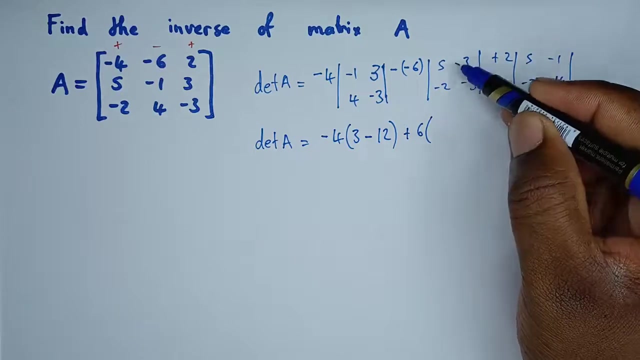 The determinant of A will be given by negative 4.. 1 times negative 3, that's 3, minus 3 by 4, that's 12.. So negative negative will give us a positive 6.. 3, negative 3 times 5 is negative, 15.. 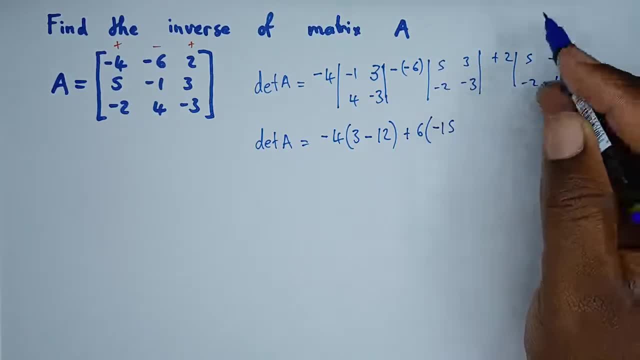 Negative 2 times 3 will give us a negative 6, then to become a positive 6, because we have to subtract the two products, Then plus 2.. 4 times 5,, that's 20.. Minus 2 times 1,, that's a positive 2.. 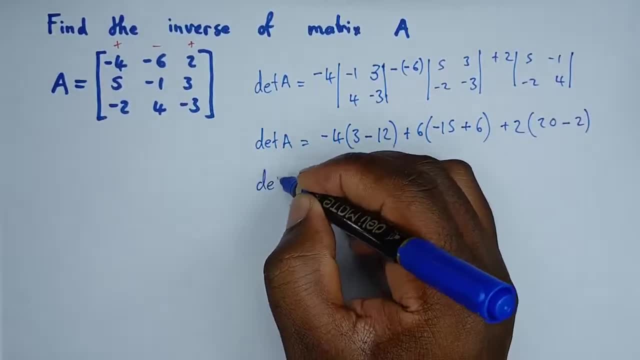 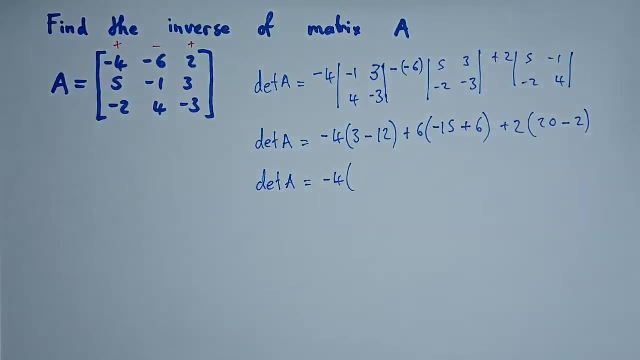 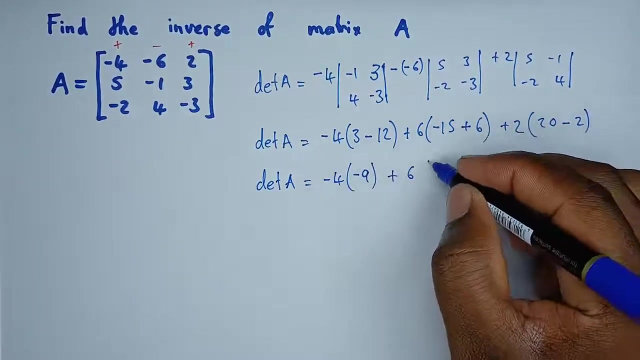 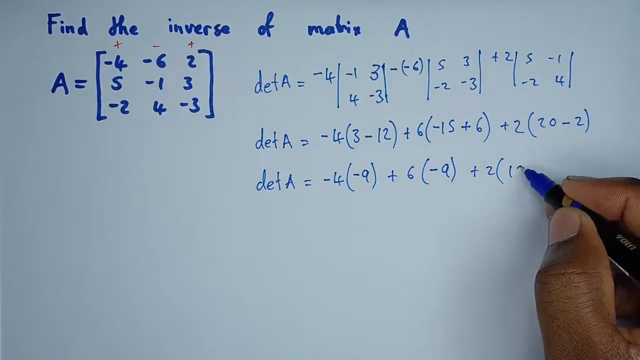 Like that. okay, So the determinant is given by negative 4 here. like that: Then 3 minus 12 will give us negative 9.. Plus 6, this will give us a negative 9 again. Then plus 2, this will give us 18.. 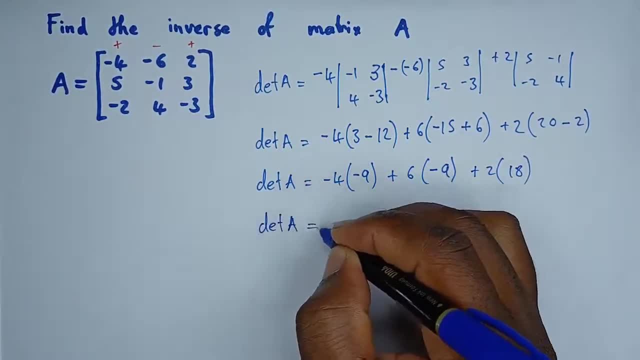 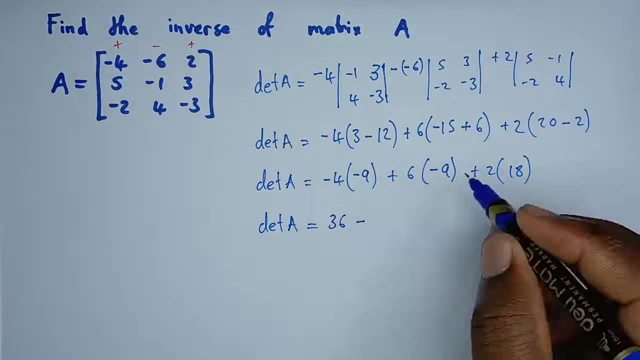 Okay, So let's continue with it. The determinant of A will be given by multiplying these two. we will simply get 36.. Minus 6 times 9,, this should give us 54.. 2 times 18 should give us 36.. 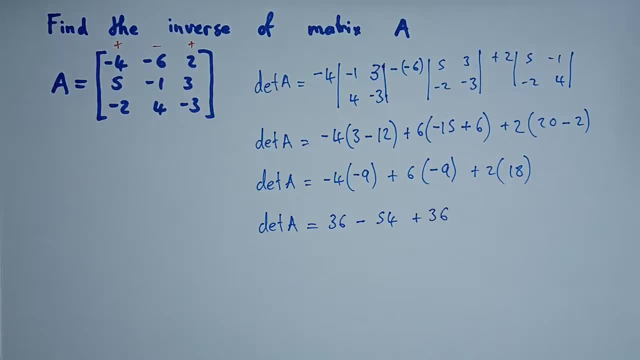 Okay, Then from there let's just add what we have. So 36 plus 36.. So let's just say determinant. So 36 plus 36, that's 72.. 72 minus 54 should give us a positive 18.. 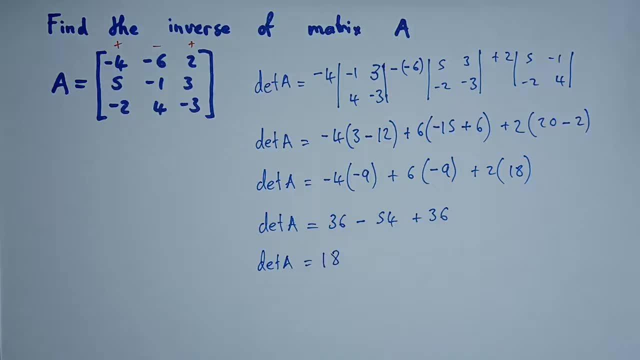 So the determinant of this 3 by 3 matrix is simply positive 18.. Okay, So we'll come back to this determinant. Let's just proceed and find the cofactor, Okay. Okay, So let's go back to matrix A. 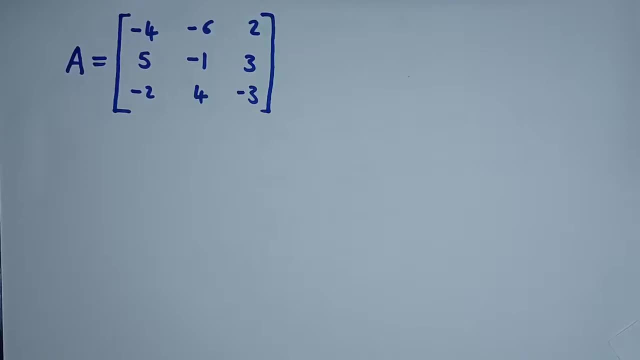 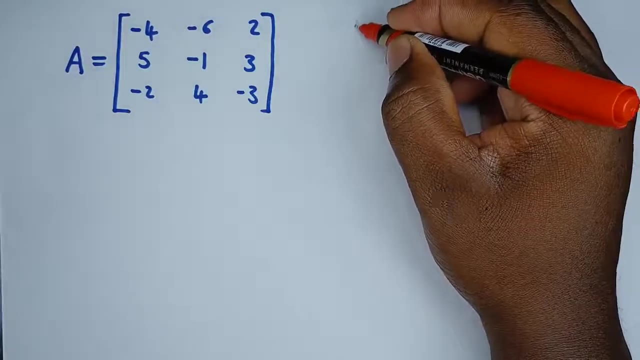 Remember we've just found the determinant so far. So now there is this sign rule that you need to know when creating cofactors. So the sign rule looks like this: If you have a 3 by 3, this is my 3 by 3 matrix. 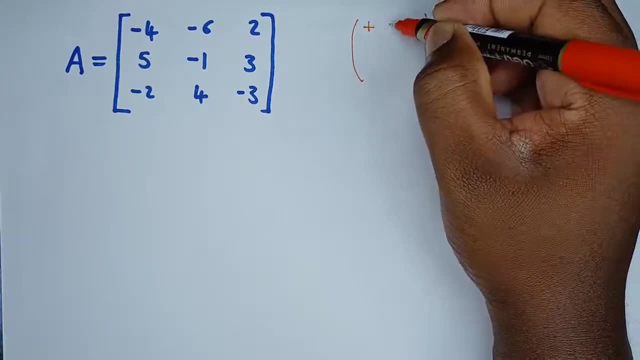 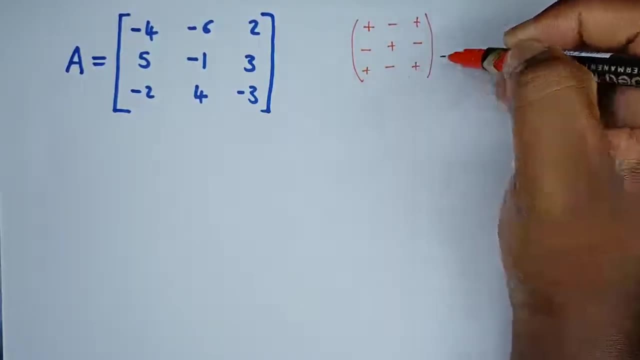 Whatever you have here is positive. What is here is negative. This is positive, Negative, Positive, Negative, Positive, Negative, Positive, Like that. So I will show you how this will come in play once we start creating the cofactors. 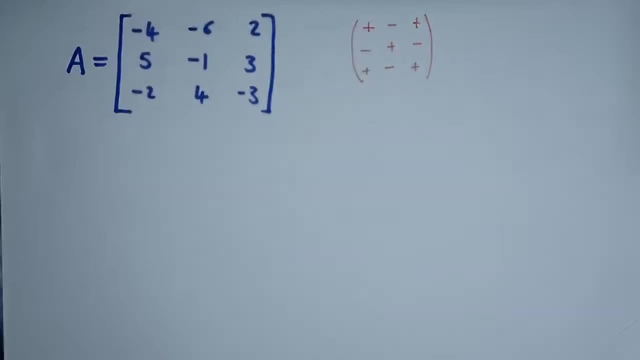 Okay, So from there we're going to create 2 by 2 matrices that we're going to use to find 2 by 2 determinants to get to the cofactor. So this is what is going to happen: I'm going to create a very big matrix. 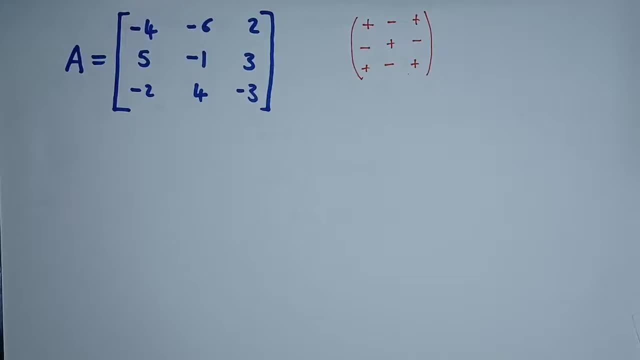 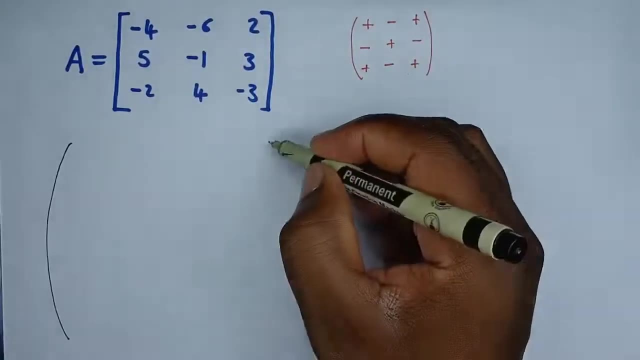 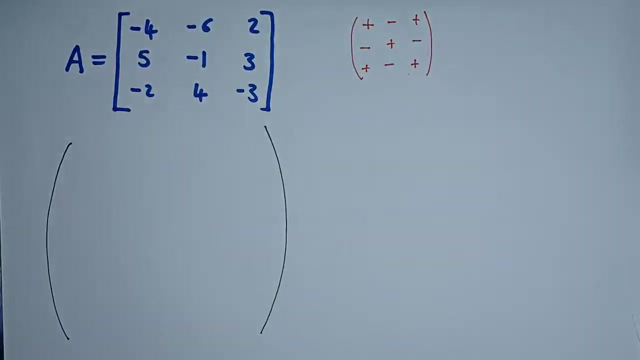 This way. Okay, So I'm going to create something very big, Something like that. Okay, Like that. So I want to create 4, sorry, not 4,, but 9, 4 by 4 matrices. So that's the first one. 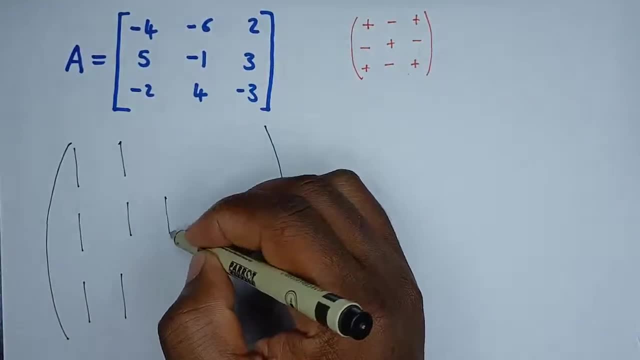 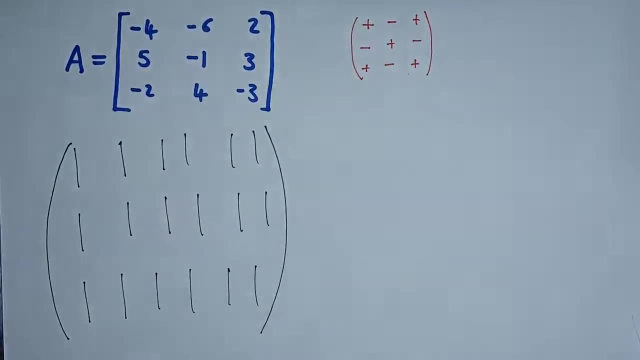 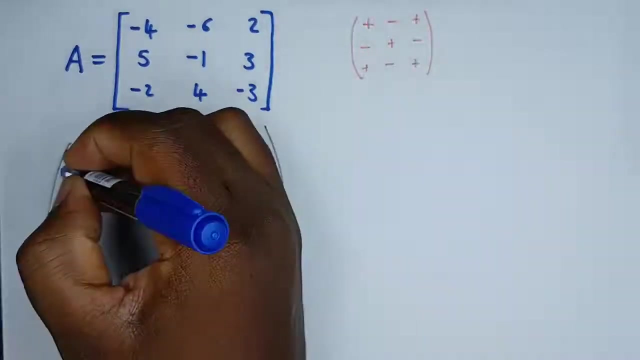 The second one, Third, Fourth, Fifth. Like that, Some of them look small. Okay, So you will see what will happen once we start replacing the intended values. So now, according to this, this one is positive, This one is negative. 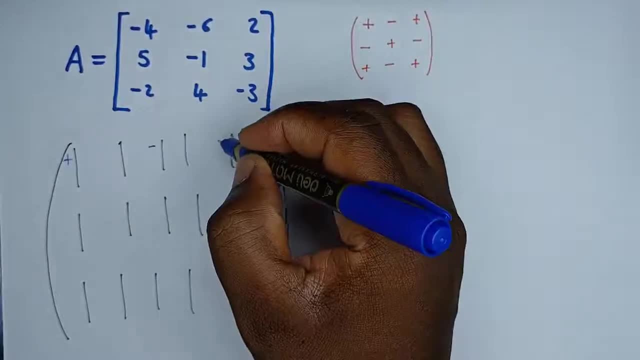 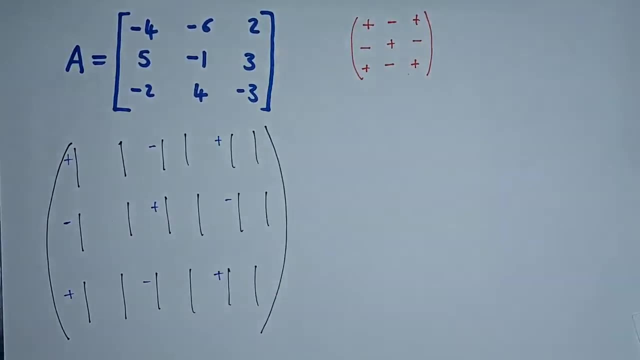 This one is too small. We'll make it bigger. This one is positive. This one is negative, Positive, Negative, Positive, Negative, Positive, Like that. Okay, So now we want to start filling in these 2 by 2 matrices with values from matrix A. 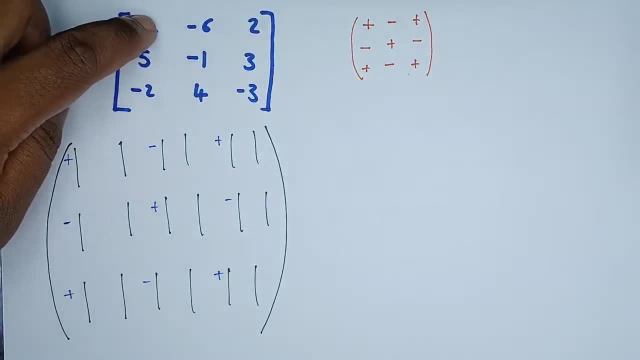 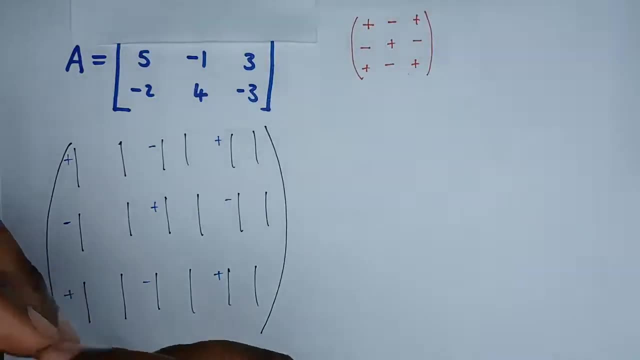 So, to start with, we'll start with this 4 here at this position, which is this position here. So everything in the row of 4. In the row of 4 should be hidden and everything in the column for 4 should be hidden. 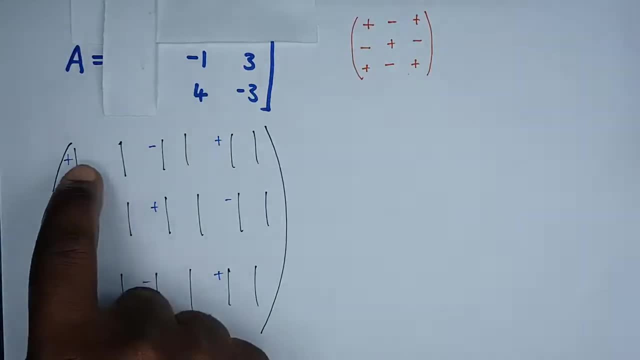 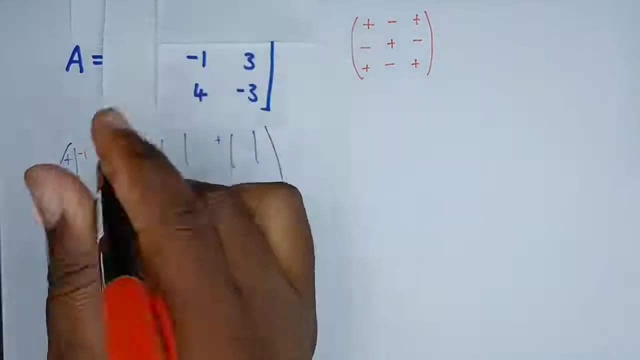 So the remaining 2 by 2 matrix is what should be put in the position for 4.. So the remaining 2 by 2 matrix is simply negative 1 according to this, 3, 4, negative 3.. Like that? 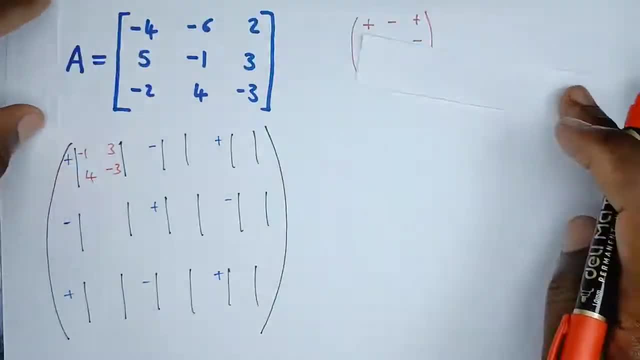 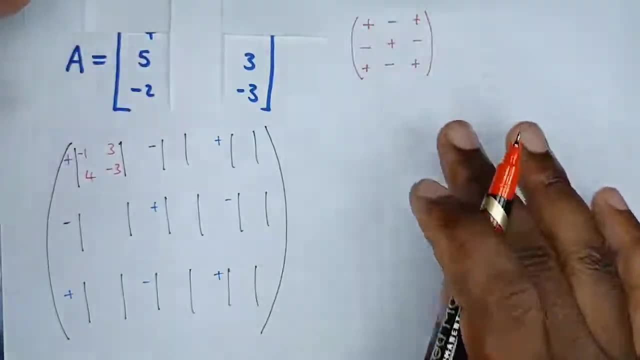 Then from there we move on to 6.. So we hide the row and column for 6.. Like that. So we'll create a 2 by 2, which is 5, negative 2, 3, negative 3.. 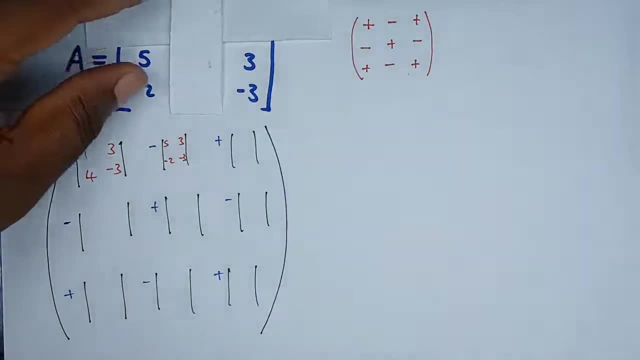 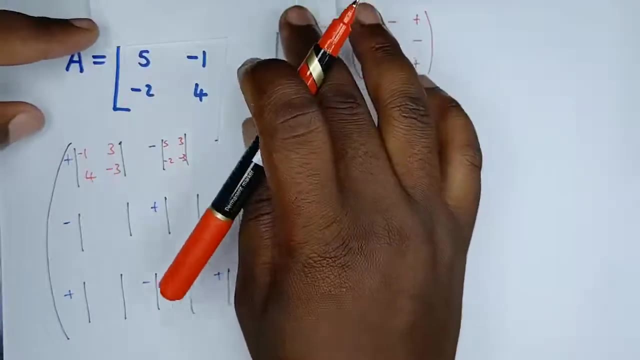 Sorry about that space there. Then the last value in the first row is 2.. So we hide the column for 2 as well as the row for 2.. Like that. So the 2 by 2 formed will be 5, negative 1, negative 2, and 4.. 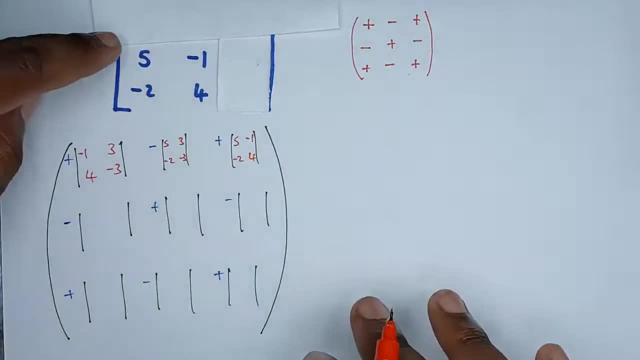 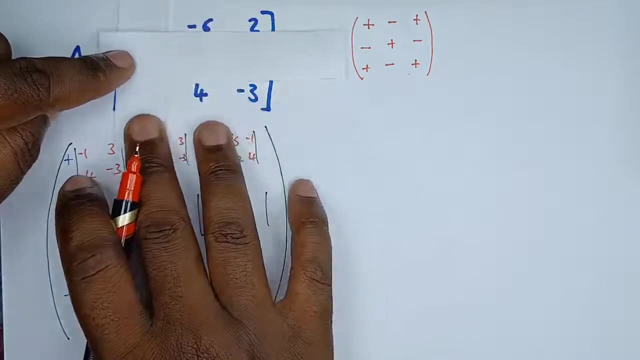 I'm sure you get the idea now. So if you come to 5, this 5 here. Okay, If it's at this position, we're going to hide its row as well as its column. So what's the 2 by 2 formed? 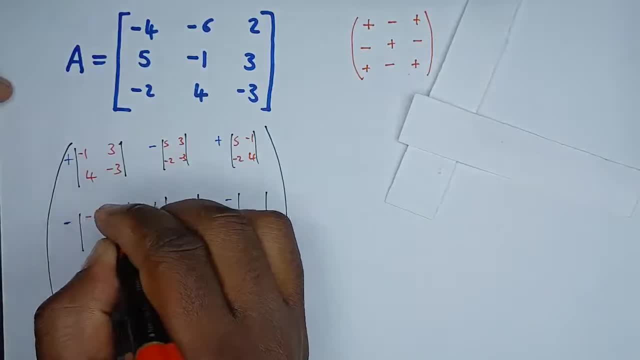 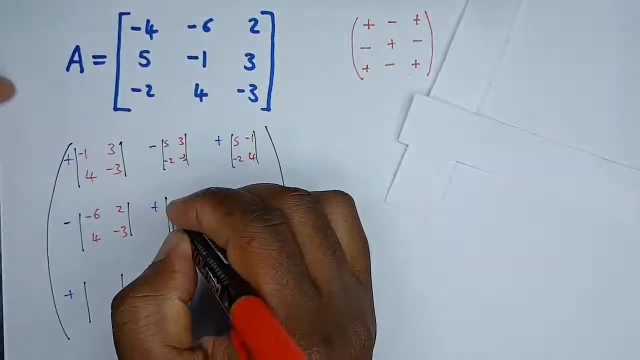 So the 2 by 2 formed will simply be negative 6, 2, 4, and negative 3.. We come at this one, we hide this and this. we'll remain with negative 4, negative 2, 2, and negative 3.. 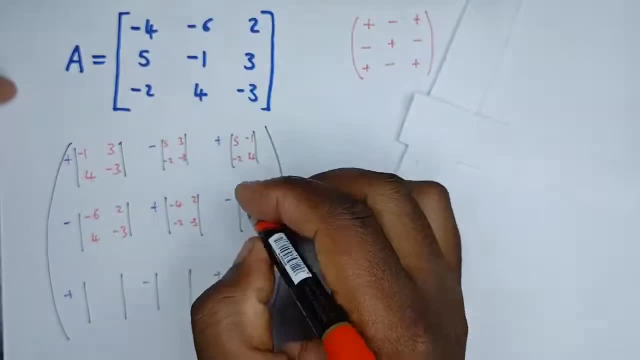 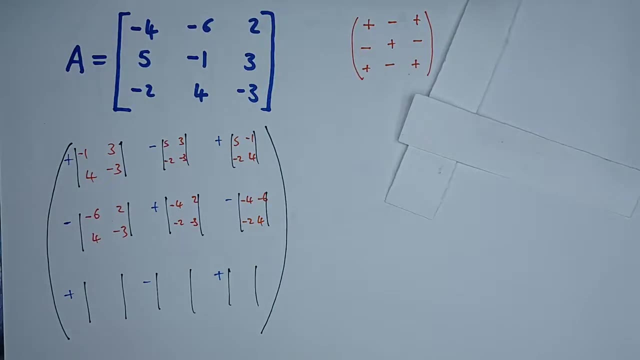 We come here, position 3, we'll hide this and this, so we get negative 4, negative 6, negative 2, and 4.. Then the last row now. So at this, position 2, so this and this, we'll remain with negative 6, negative 1,, 2, and 3.. 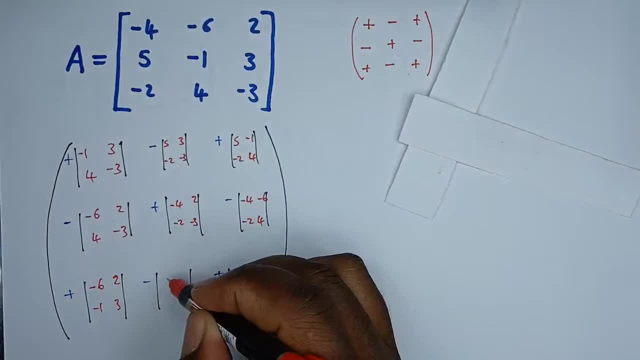 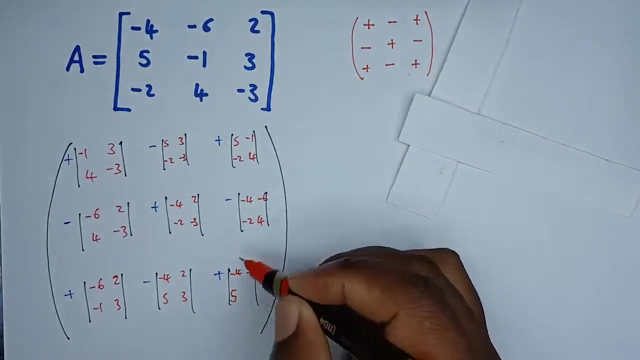 If we come at this position, so it's this and this, so negative 4,, 5,, 2, and 3.. At this position, it'll be this and this, leaving us with negative 4, negative 6, and negative- not really negative 2, but 5 and negative 1.. 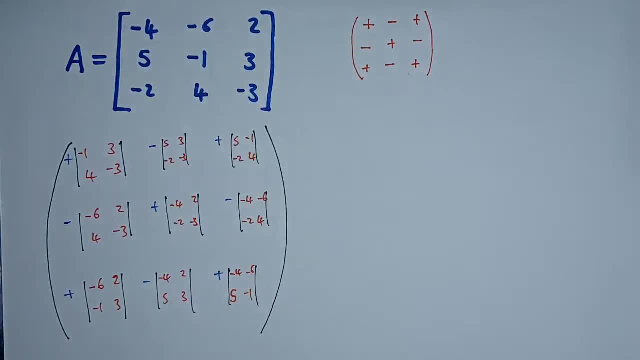 Okay, So now, with these values, we can create the core factors. now We're going to find the determinants at every position. So of course, the determinant is by multiplying this minus that, Then that will be giving us the determinant of each of these 2 by 2 matrices. 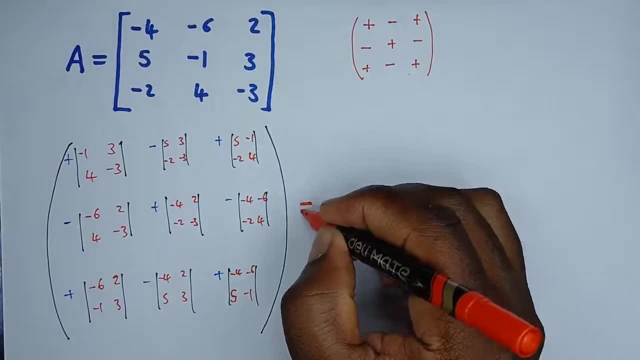 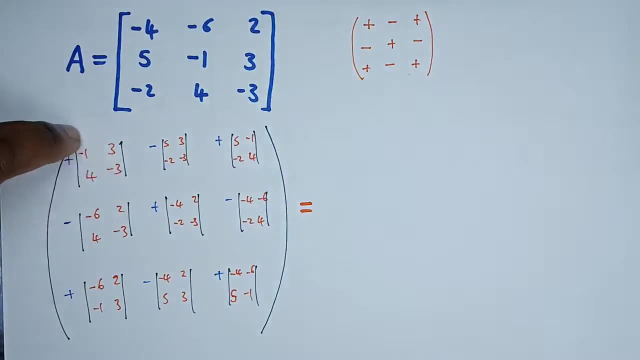 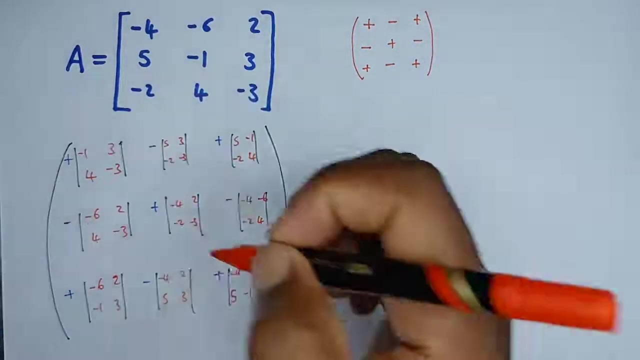 Okay, So let's create. let's create the core factors. So, to start with here, we're going to get 3 minus 12.. That's 3 minus 12 to give us negative 9.. So at that position we'll have negative 9.. 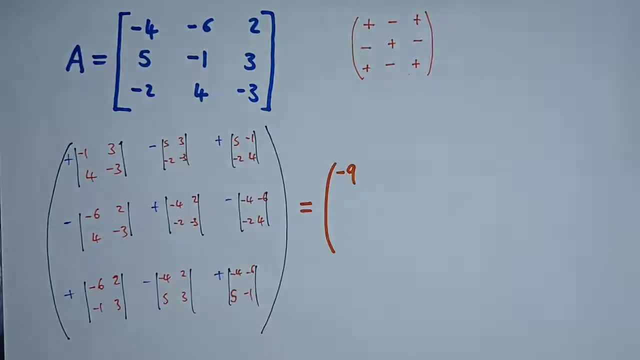 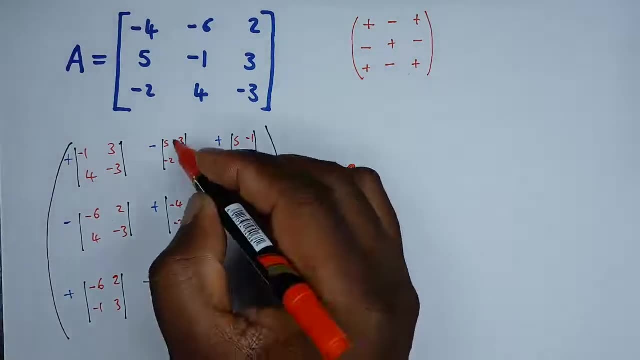 At this position, we'll have negative 15, negative 15 plus 6,, which is negative 9.. So we get a negative 9, but there's a negative, hence it becomes positive 9.. 5 times 4,, that's 20.. 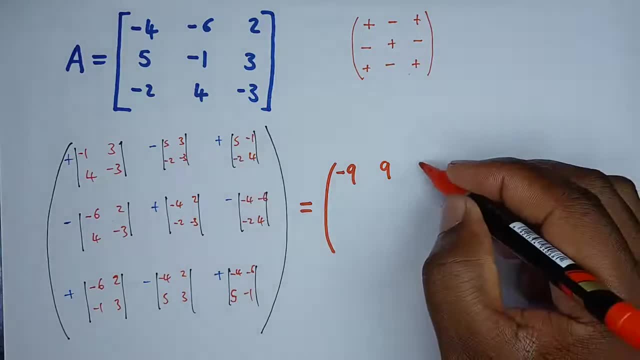 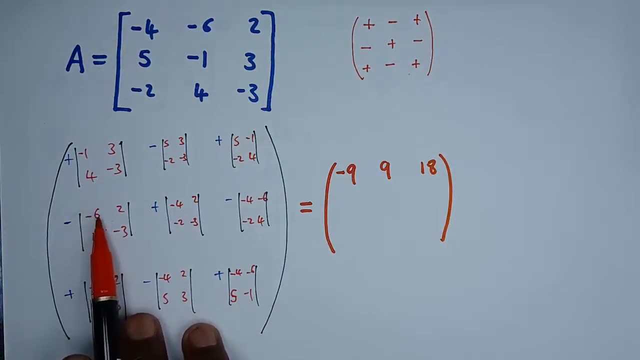 20 minus 2.. 20 minus 2 will give us 18.. Okay, If we come at this position, negative 6 times 3,, that's 18.. So 18 minus 8 will be 10.. Now there's a negative outside, so we have negative 10.. 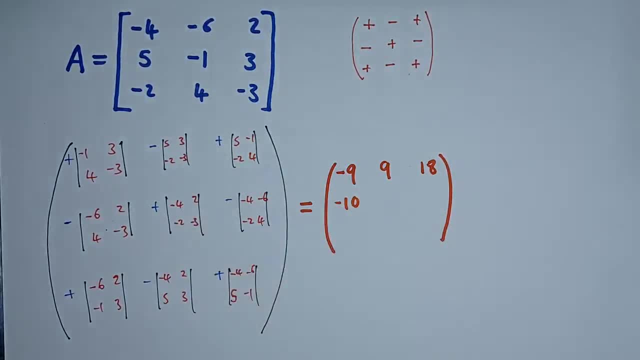 4 times 3, that's negative 12.. Negative 12 plus 4 should be negative 8.. Okay, If we come here 4 times 4, that's negative 16.. Negative 16 minus 12 should give us a negative 4.. 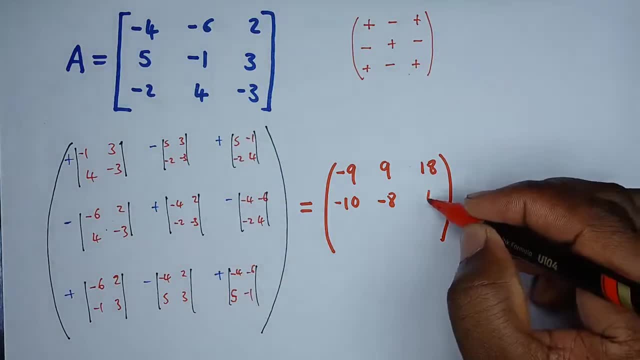 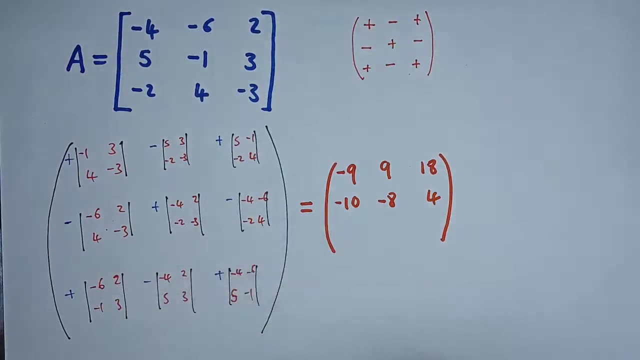 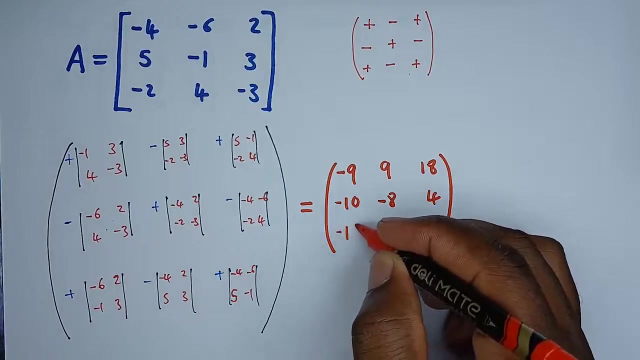 Negative 4, there's another negative, so it will give us a positive 4, like that. Then at this position we'll have negative 18.. So negative 18 plus 2. Which will give us negative 16.. Like that. 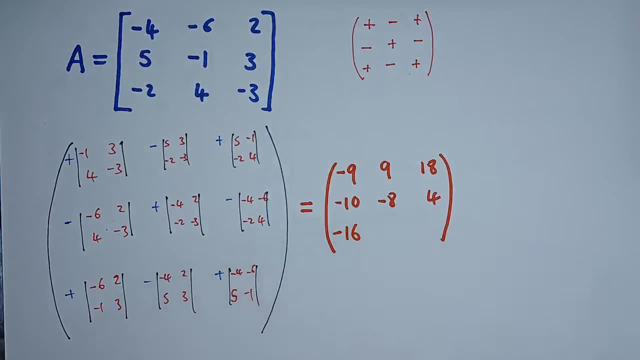 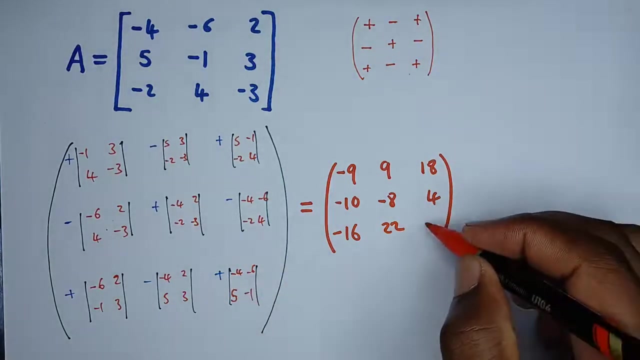 Here we'll have negative 12 minus 10. Which is negative 22. So there's a negative here. it will become positive 22.. Like that, Then negative 4 times negative. 1 is 4.. 4 plus 30 should give us 34.. 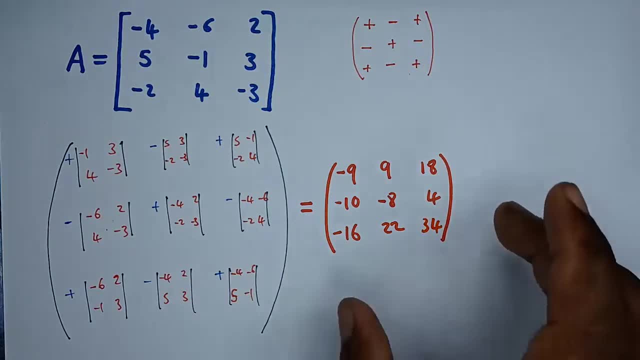 Like that. Okay, So what we have here? the core 4.. So, with these core factors, what we're going to do is we're going to transpose this matrix. If we transpose this matrix, what we're going to get is the adjoint of A. 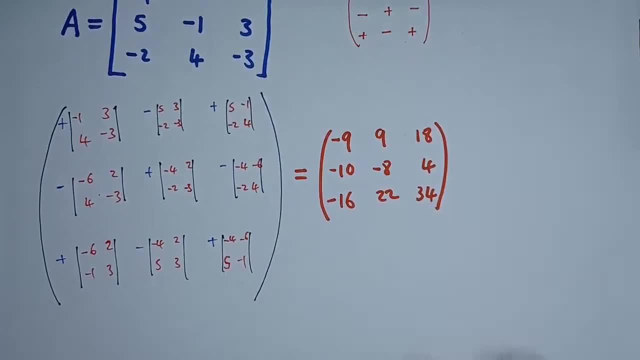 So, after finding your core factors, we have to transpose it. So let's transpose. So transposing this matrix gives us the adjoint of A, So adjoint of A, Adjoint of A will be given by the transpose of this matrix, of course. 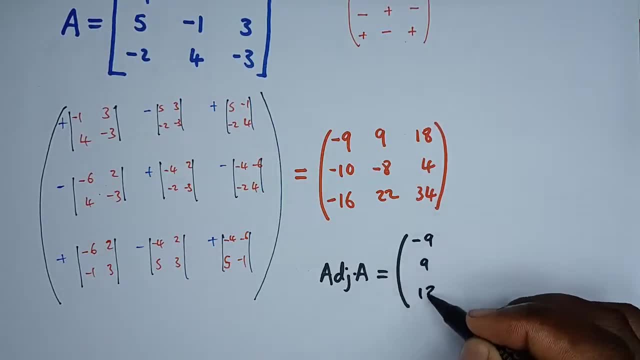 So if we transpose this, we'll get negative 9, 9, 18.. Negative 10, negative 8, 4.. Negative 16, 22, 34.. Okay, So this is our adjoint. So now we're going to use the adjoint as well as the inverse to find the 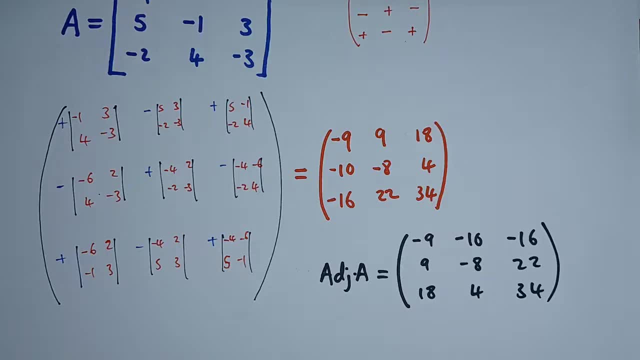 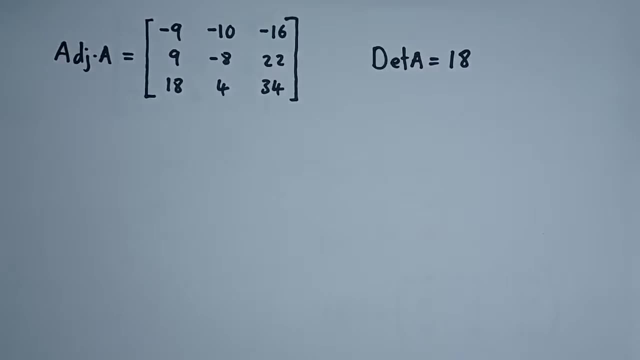 Sorry, The adjoint and the determinant to find the inverse. Okay, So this is what we've achieved so far. We've managed to find the adjoint by using core factors, transposing the core factor as well as the determinant that we found in the first step. 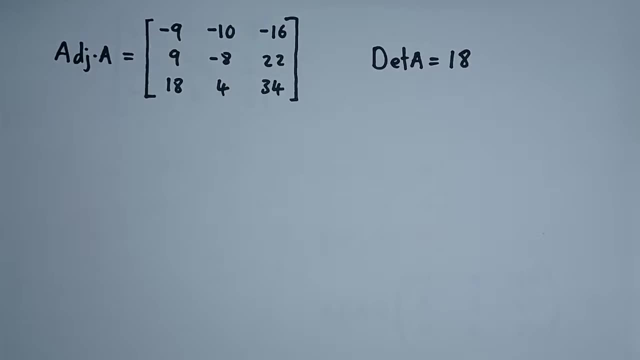 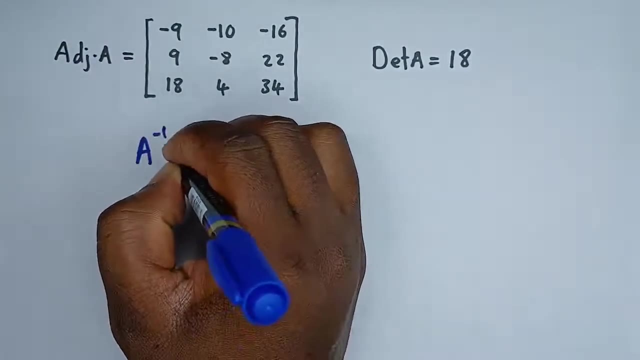 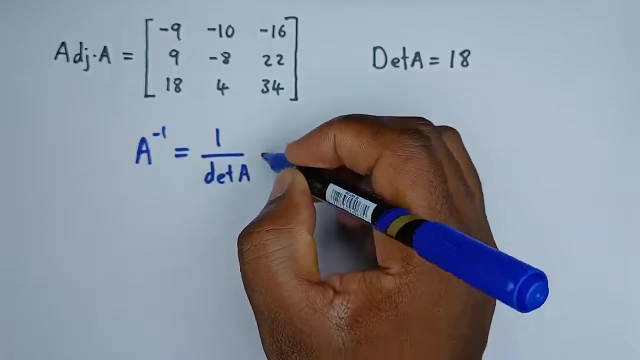 So now that we have these two, we can proceed and find the inverse matrix. So the formula for the inverse is given by: So the inverse of A is equal to 1 over the determinant of A multiplied by the adjoint of A. 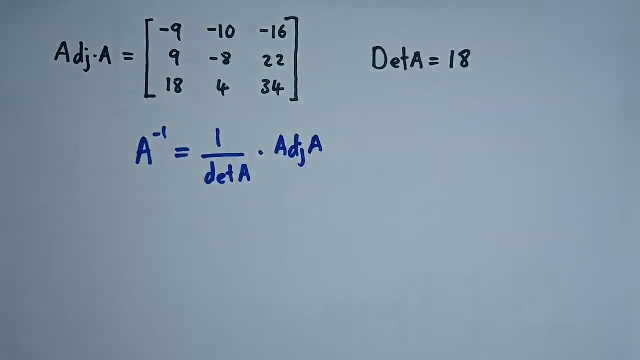 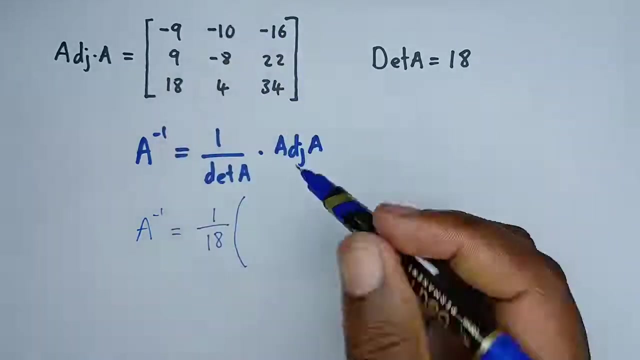 So once you multiply these two, then you get the inverse. Okay, So let's do that. The inverse of A will be equal to 1 over, Remember the determinant is 18.. Then the adjoint, which is this matrix here, is negative 9.. 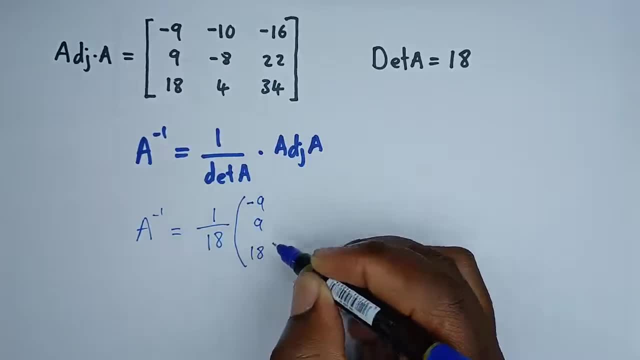 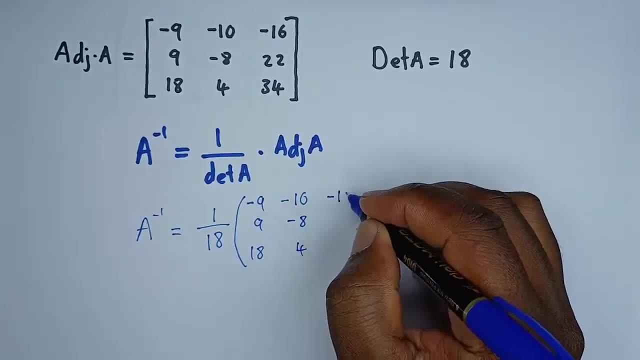 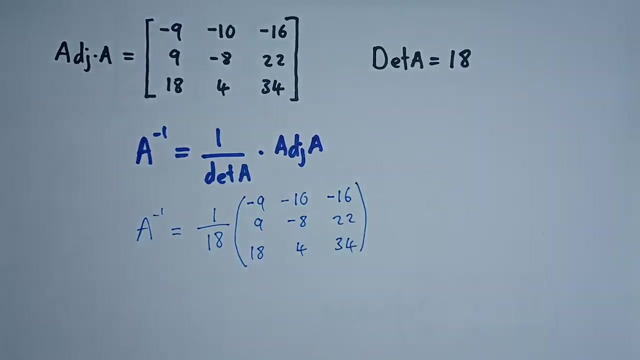 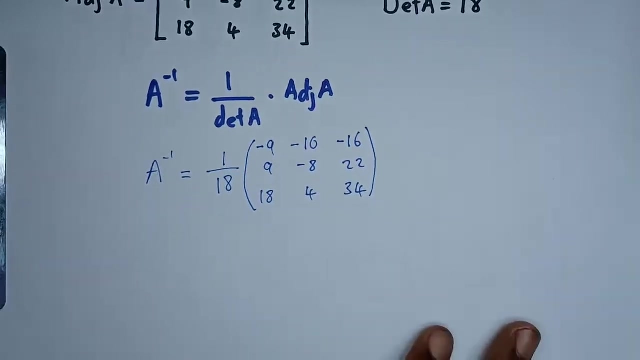 9, 18, negative 10, negative 8.. 4 there negative 16,, 22, and 34.. That So we can multiply everything inside the matrix with 1 over 18.. Or rather, we can just divide by 18.. 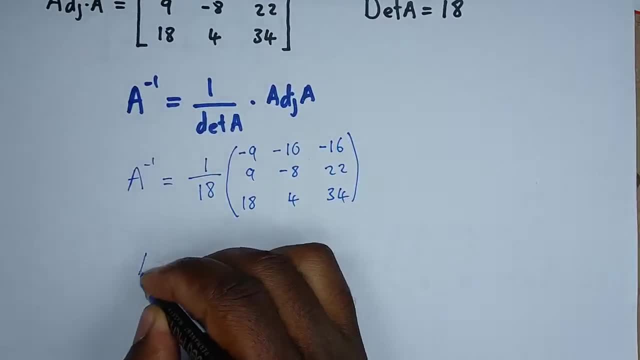 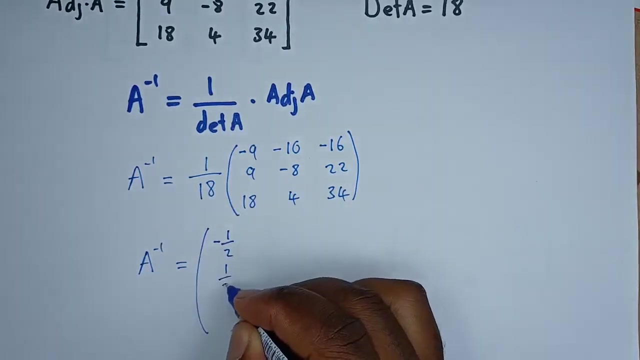 It's the same thing. Okay, So the inverse will be given by: So negative 9 over 18.. I'll just write it like this: Negative 9 over 18 is the same as negative half 9 over 18 is the same as half. 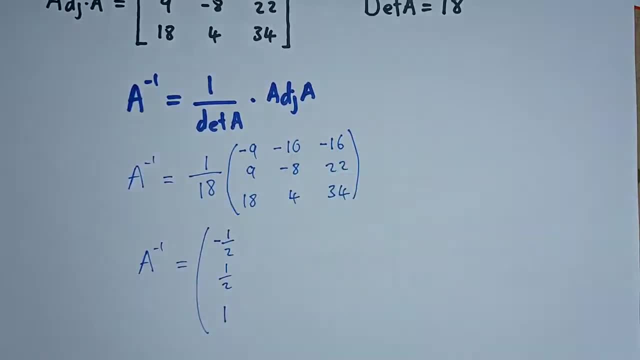 18 over 18 is just 1.. 10 over 18 can be reduced to 5 over 9 if we divide by 2. So it will be negative: 5 over 9.. 8 over 18 is simply negative: 4 over 9.. 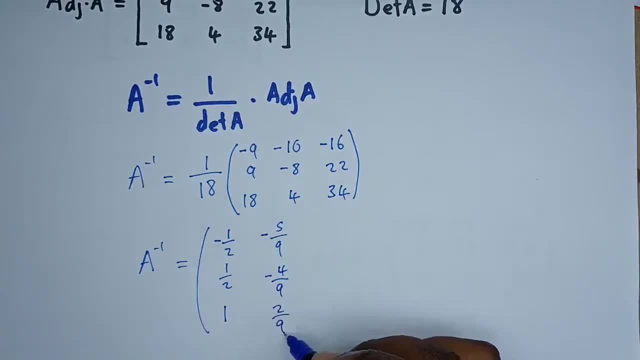 4 over 18 is simply 2 over 9.. 16 over 18 will be 8 over 9, negative 22 over 18 can be reduced to 11 over 9.. Then 34 over 18 can also be reduced to 17..